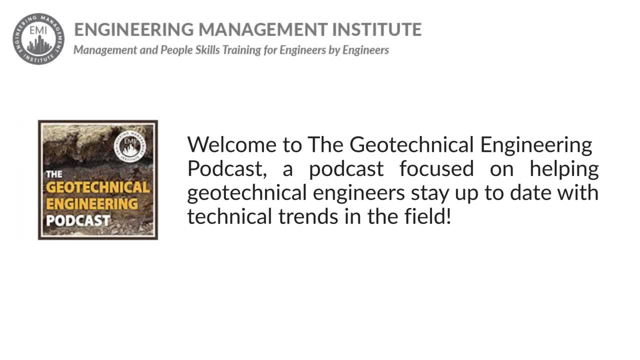 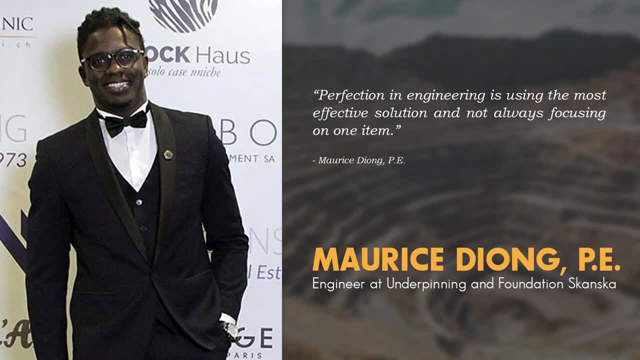 Hello and welcome to the Geotechnical Engineering Podcast. In this episode of the Geotechnical Engineering Podcast, I'll be talking about Maurice Diong, PE, an engineer at Underpinning and Foundation Skanska. We'll be talking about deep foundations And I'm your host, Jared Green. 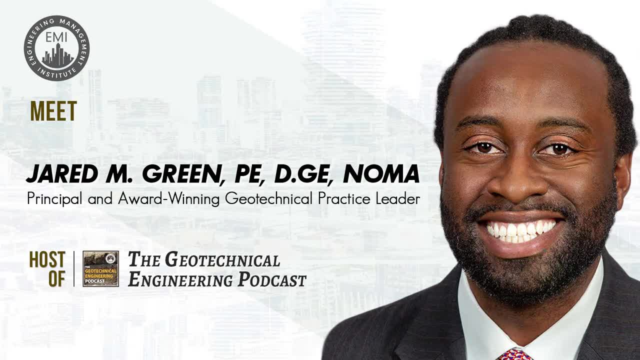 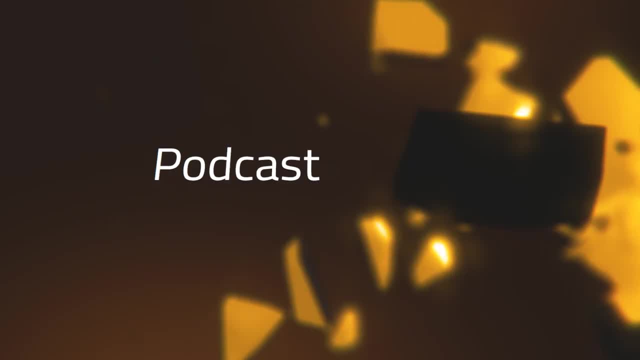 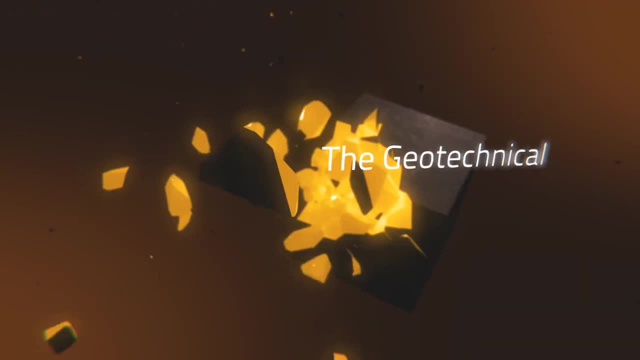 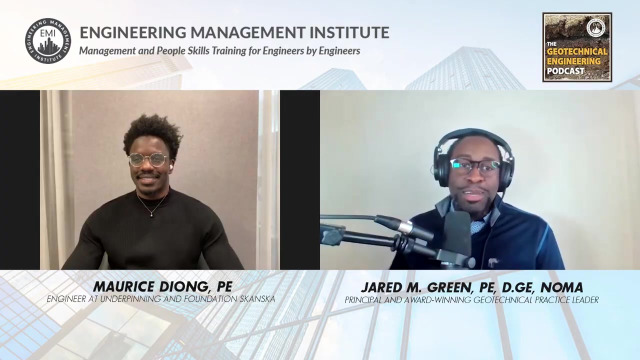 and this is the Geotechnical Engineering Podcast, a podcast focused on helping geotechnical engineers stay up to date with technical trends in the field. And with that, let's jump right into today's episode. Maurice, welcome to the show. How are you doing, man? 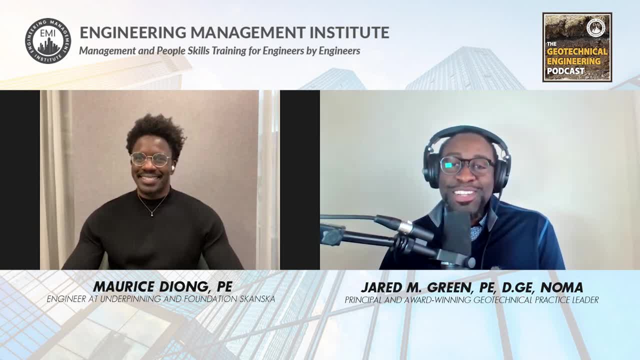 I'm doing great, Jared. Thanks for having me. No problem, I appreciate you being on here. I was really looking forward to our conversation. It's been a while since we've talked, but I'm glad that you could be here with us. 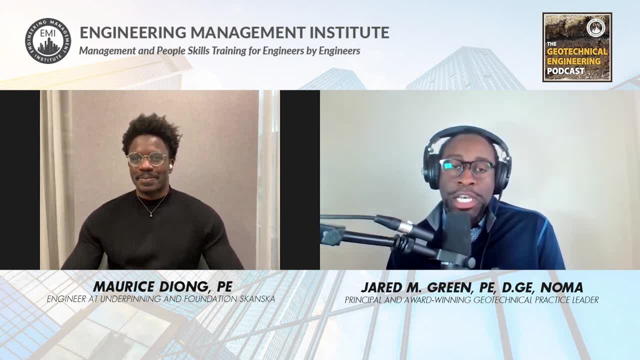 All the pleasure is mine, Excellent, Excellent. So I'd love it if you could tell us a little bit more about your career journey to date, And also tell us what is it you do on a daily basis. Well, so it all started. during my last year of college. I got an internship with Underpinning. 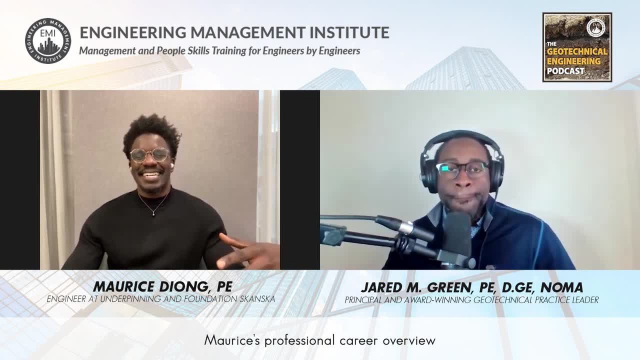 and Foundation Skanska. Sorry, Yes, Okay, No worries, And then yes, And then I did a. they have a small rotation program, So during that rotation program you would jump from, you would do estimating, you would do engineering. 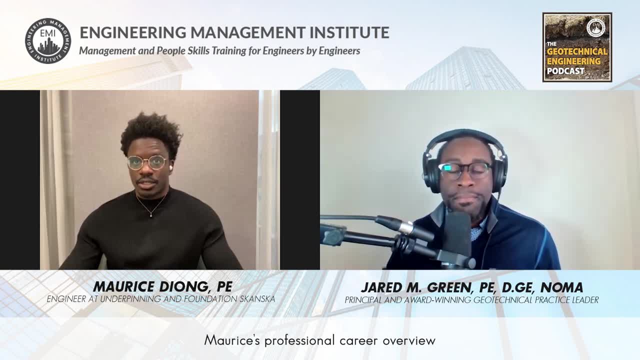 design, operation, safety and cost control. So I did a little bit of that And by the time my internship ended I got a job offer with Underpinning And, yeah, I stayed with them. So I'm part of the design team And so what I do is submittals, sometimes in-house. 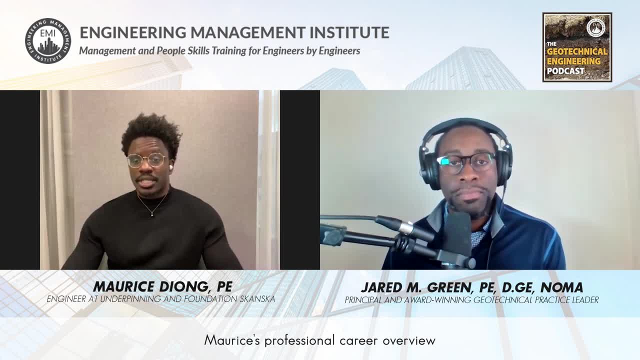 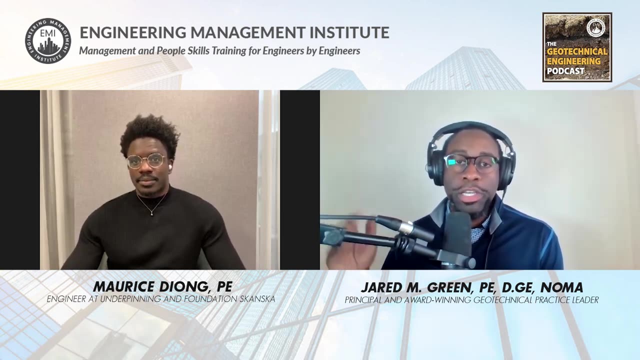 sometimes some design. I help operations set up jobs. At this very moment, for example, I'm doing some estimating And at times when they need me, I actually go to the job and I run the job. That's awesome, And so the place where you got your internship, that's where you're working. 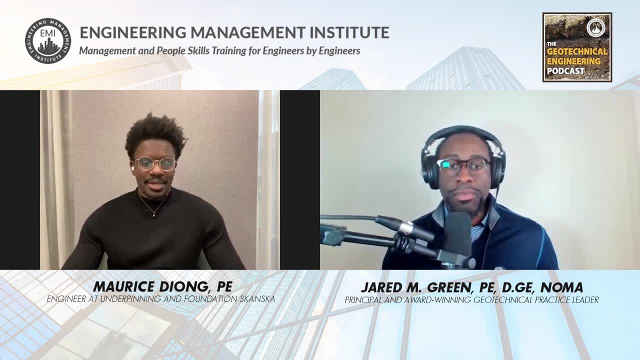 full-time. That's where I'm working full-time. And, yeah, like I said, I do a little bit of everything. So even when I send an email these days, my signature says engineer, Because I was like: okay, what am I? I'm still an engineer, I'm going to be an engineer. I'm going to be an engineer. 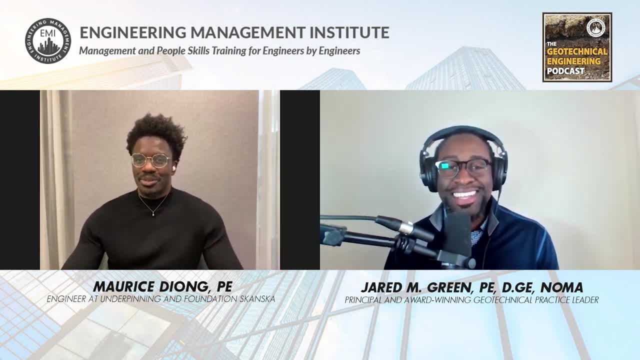 I just signed engineer, since I do a little bit of everything- Excellent. Well, I talked to a lot of listeners that are thinking about getting an internship And it's great to hear what you just said, because I can't stress it enough: When you get an, 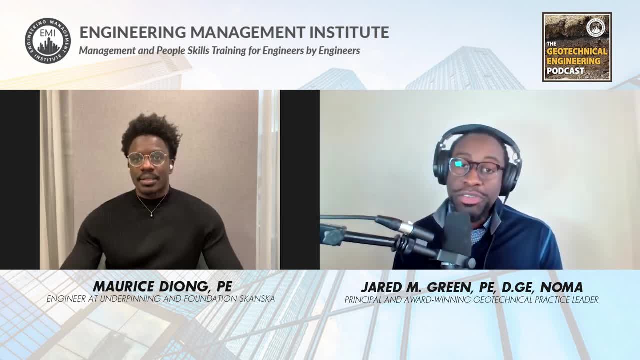 internship. that can be the start of your career. There are internships. you intern and you say, well, I never want to do that again, And you kind of change or change different company or different field. But there's a lot of times where I guess you go to the internship, you like what you're. 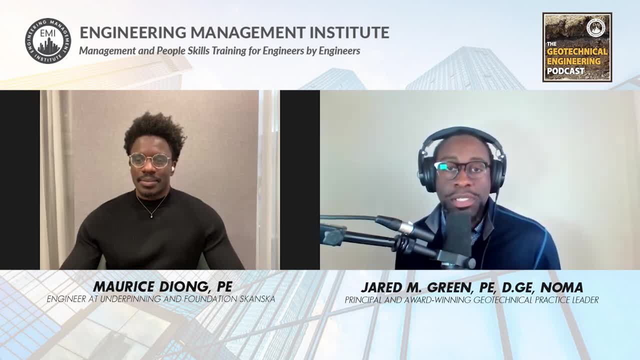 doing They like, having you there and you get an opportunity to do that And you get an opportunity to work full time. So that's awesome. That's awesome, Thank you. Excellent And I understand because I work with your company quite a bit And I understand you. you're involved with deep 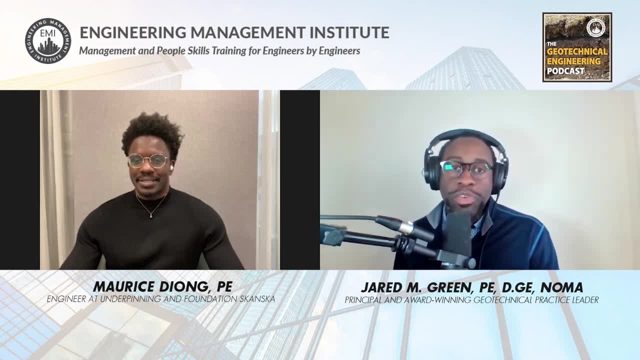 foundations. I'd be curious to hear a little bit more about the types of deep foundations you work on, So the ones you design and things of that sort, And there might be listeners that have no idea what deep foundations are. They could be early in their studies, So it'd be great if you 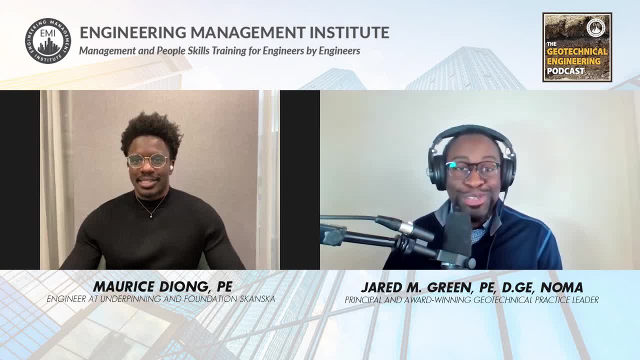 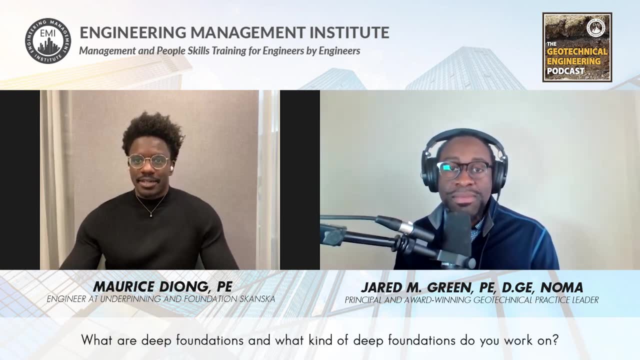 could tell us more about what deep foundations are, why they're used and what types there are. All right, So again, back in college, I had the deep foundation, the DFI scholarship. So the DFI is an international association for all entities involved in deep foundations. right, So it could be from. 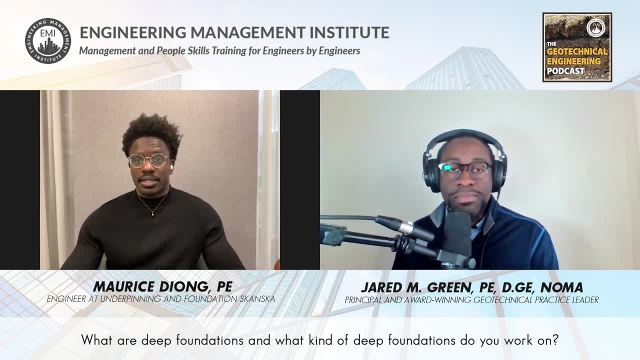 the design and or the construction of the foundation and excavation. So all those companies you know get together and are all part of that association. So another question is: what is deep foundations? Well, sometimes you cannot do the typical shallow foundation when it comes to a building. right For the listeners who don't. 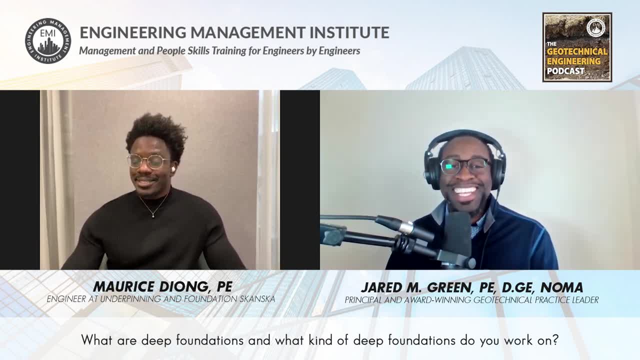 know what the foundations are. it's the part of the building that nobody sees, but also the most important part of the building. So yeah, so sometimes you can't do a shallow foundation, you can do a footing, you can do a mat, So you use piles right. 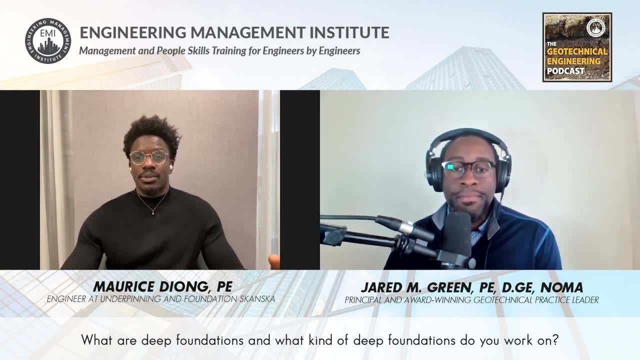 So you drill or driven and you install them into the ground So those elements provide some load capacity through bearing or friction. So I focus on micro piles, which are small diameter piles, And I think that's the only thing small about them, because it's, you know, setting up. 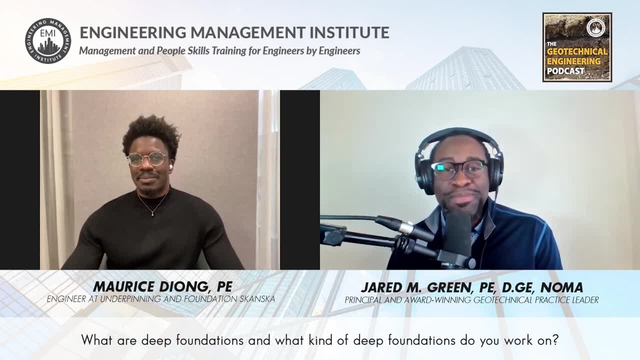 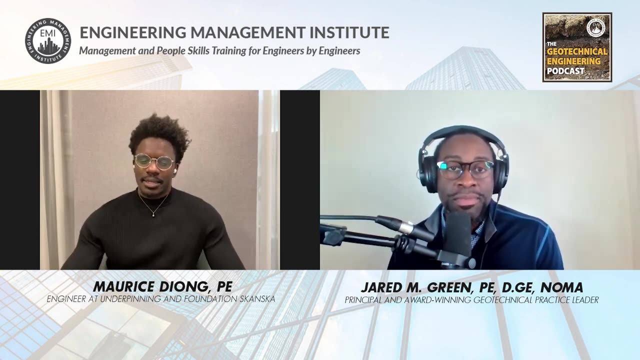 is pretty complicated And there's a lot that goes into it. Excellent, excellent. And you know, for context, what diameters are you usually looking at, Like what's the smallest diameter that you've seen on a job? Well, I usually focus from, I think, anywhere from six inches to, I'd say, 13 and three eighths. 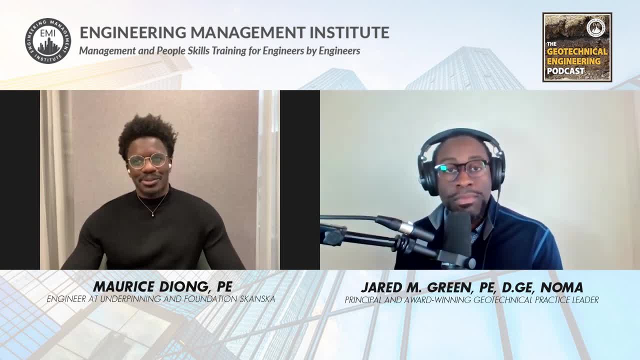 Okay, But these days, I mean, people tend to push the envelope a little bit and you end up having like 18 inch micro piles. Okay, got it. But I like when it's around 12, 11 inches, Okay. And then for you, I mean, are you doing limited access work or your work is still outside? 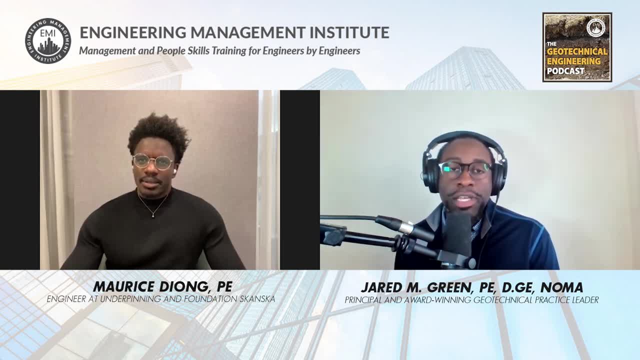 By outside? what do you mean? I mean like: are you doing anything inside of like exist? like when I think about micro piles or mini piles. sometimes it's inside of an existing building or you have to go in through a facade. 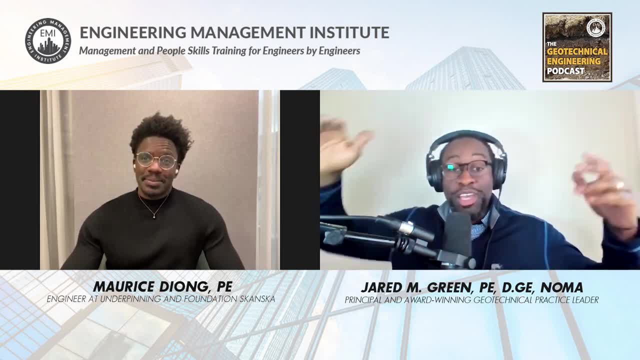 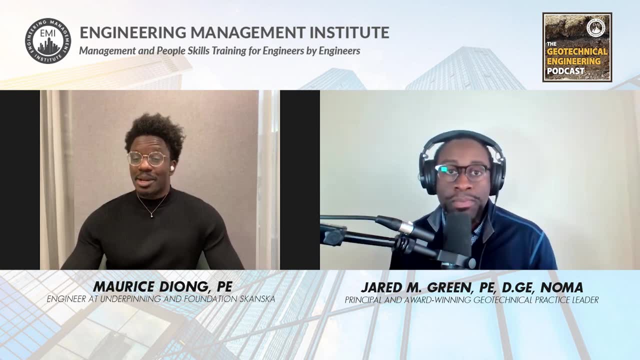 with a small rig. Then there's other times where you have an open field, you have plenty of headroom and you're still using small diameter elements. But You know, whenever we have an open field, I'm actually happy, Like yeah, it's open, It's. 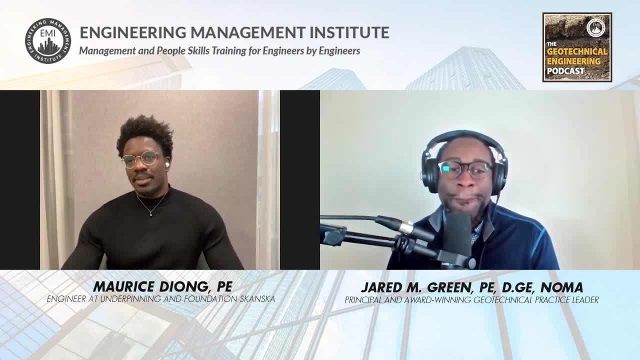 Christmas We're going to have a good time, But no, I mean being in New York City a lot of time. we have not a lot of headroom, so no headroom. And yeah, I mean we got to work with what we have. 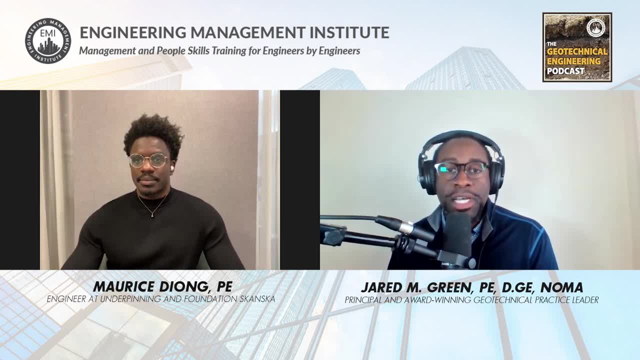 Got it, Got it. And then there's a lot of different types of construction techniques for deep foundations. I'd be curious to hear a little bit more about those. You know, what are you seeing? What's on the horizon? Well, I mean, like you said, you know you have a lot of different types. right, You can drive them. 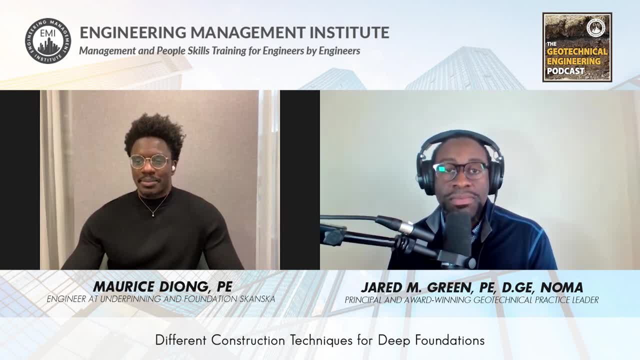 you can drill them, you can jack them, You can even screw them right, And it really depends on the soil conditions, on the physical constraints that you have. Like I said, I focus on micropiles. So for micropiles you can you have 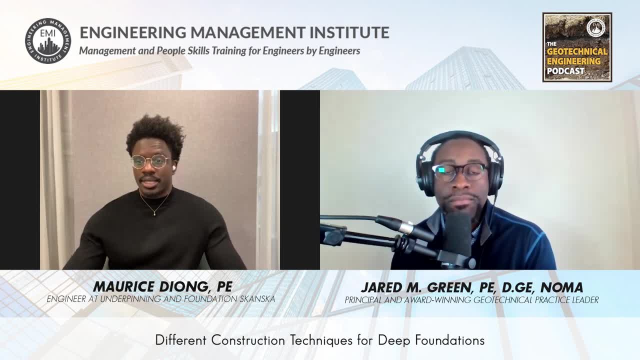 I mean you have different methods, right Could be rotary, could be. you can use a down-the-hole hammer duplex system: overburden. You have a lot of different ways to do it, And they can even use a down-the-hole hammer water flush, which was interesting. 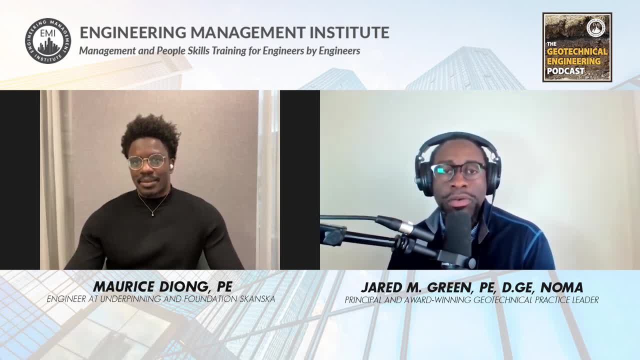 When are you using a system like that? What type of geology would make you go that route? Actually, we have not used a lot of it, or actually we've never used it. We use air flush. but I was just reading a. I was reading a paper by Donald Cruz and he mentioned it, So I actually 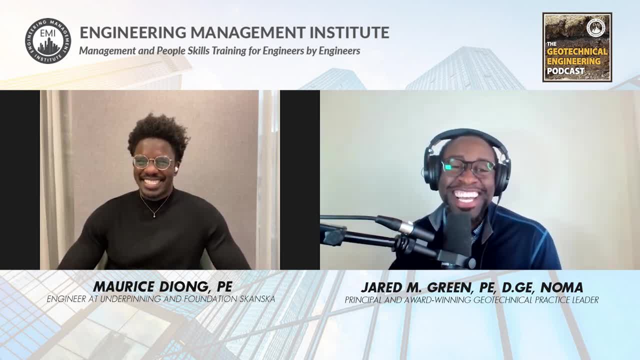 I called him to talk about it. Yeah, Yeah, There you go, And I'm sure he loved talking about it. I've heard him many times, especially at DFI conferences. Yeah, All right. Well, I'd love to hear about a Deep Foundation project that you've worked on, and how did it work? 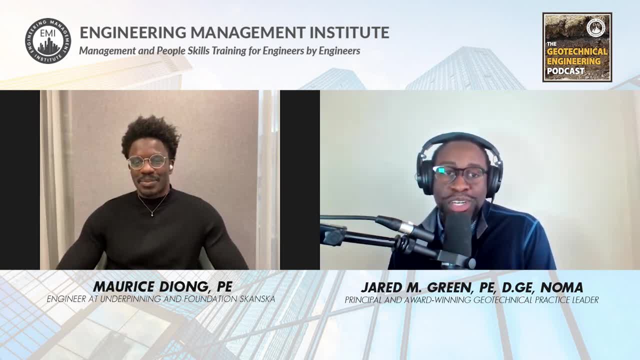 Yeah, You can have a conversation with Dr Joeığı, All right. Well, I'd love to hear about a Deep Foundation project that you've worked on, and how did it work and how are you on the field? Yeah, Yeah, Yeah, that would be fine. 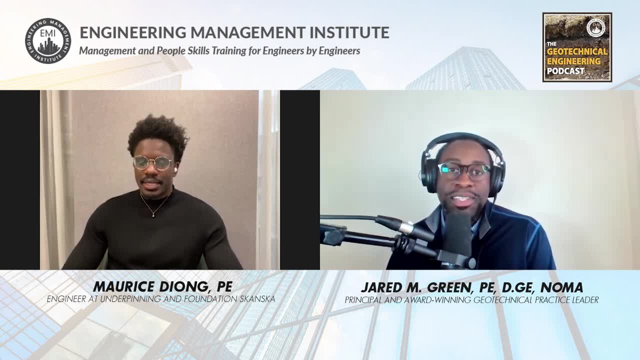 Yeah, that would be fine. Yeah, Yeah, That would be. that would be fine. how did it benefit your career? Well, there is one project that comes to mind, And so I was working on it with a former colleague of mine, Matt Bertucci. 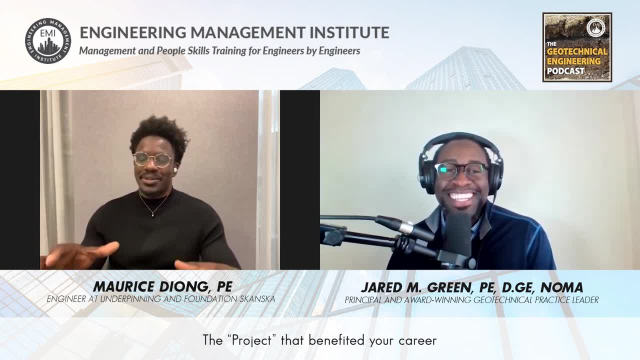 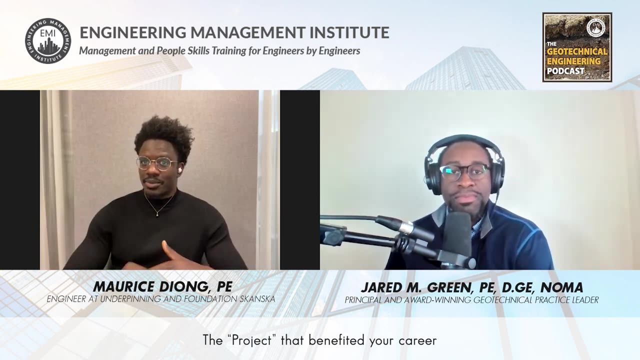 And so it's a mind blowing project. Picture this: right You are in the middle of Manhattan, right Midtown, And there is a 50 storey building that the owner wanna, you know, demolish and turn into a 70 storey building. 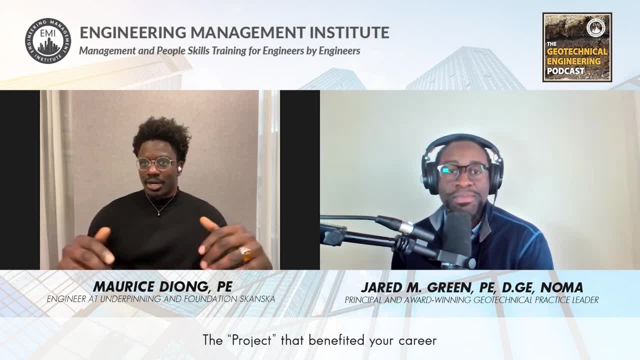 But while he demolishes the building, you are in the basement retrofitting the foundation. right, You're installing 400 micropiles in the basement, middle of New York City, You have Metro North right next to you and in the middle of the pandemic. 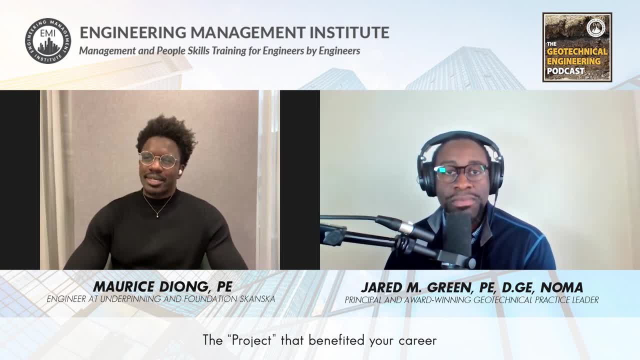 So I think, yeah, that project is one of the most impressive project I've worked on and I learned a lot. right, I learned a lot when it comes to, I think the first thing would be planning right. So there's this thing that I say. 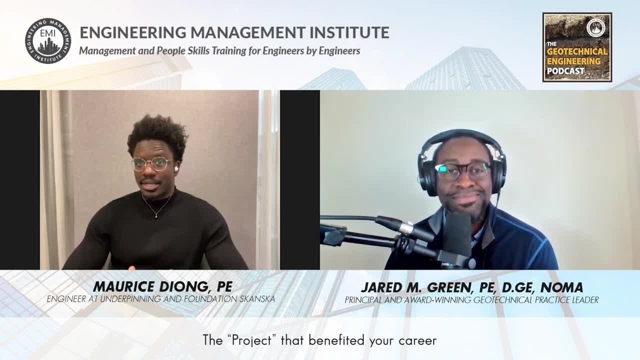 planning is underrated, but the plan is overrated, right, And what I mean by that is a lot of time. yeah, we spent some time planning, but we don't realize how important it is. It's so important to actually sit down. 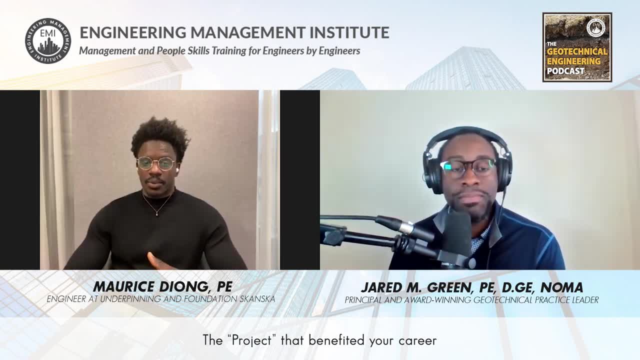 and in this project, for example, we, you know, before the job started, we got together with like a lot of great minds, right Like Teddy Salvella, our VP, Andrew Burns, and we're just talking about the project. 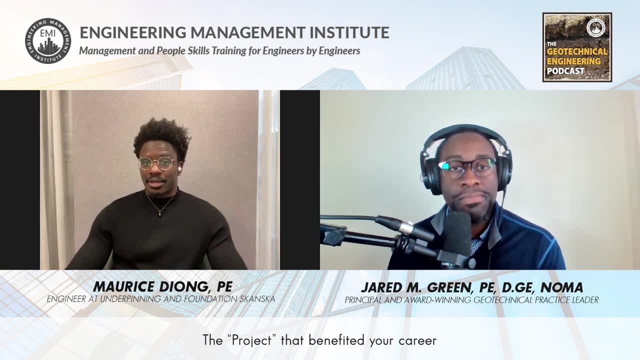 Okay, this is what we're gonna do. So it was very complicated on paper, but we got it done and we're very excited. The minute we got onto the job site, everything changed. Everything changed right. So then you wonder: what's the? you know? 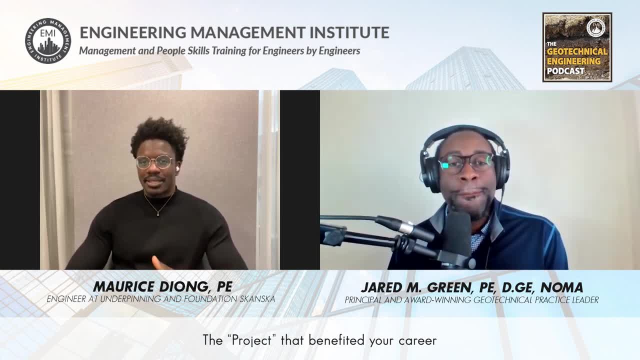 why do you need to plan? Why do you need to plan? Why do you need to plan? Well, the thing is, you know, during that planning phase we actually look at a lot of different scenarios And when you get to the site, if something changes, 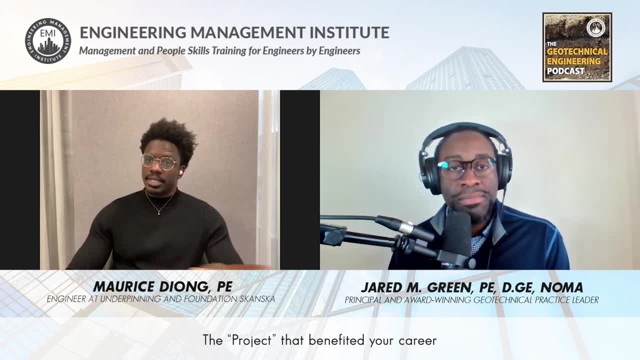 you know, it's easier for you to adapt and to take a different route. Now, why is the plan overrated? It's because, yes, you spent some time, you got a plan, but then the plan can change at any moment. 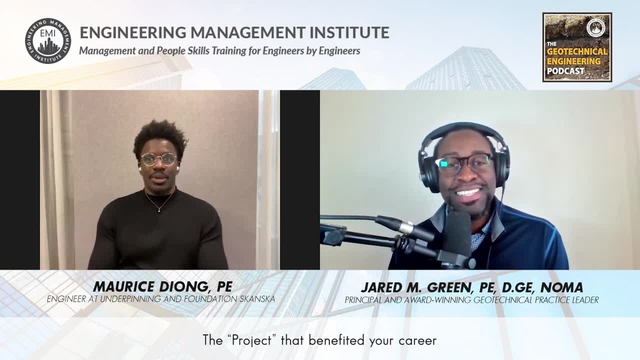 So don't just focus on it. Don't just say: well, we have to stick to the plan. No, If the plan is not working, that's fine, Let's do something else. Just stay focused and remember what the ultimate goal is. 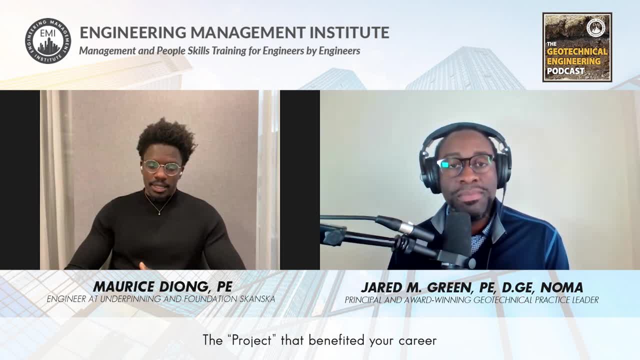 So that's one of the things I learned. The other thing is teamwork right. So when we are over there, we all want the job to be done, We want it to be done well, And you have different parties, So it's not like: well, I'm the contractor. 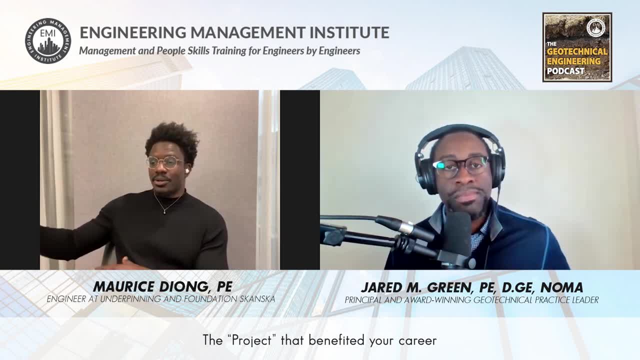 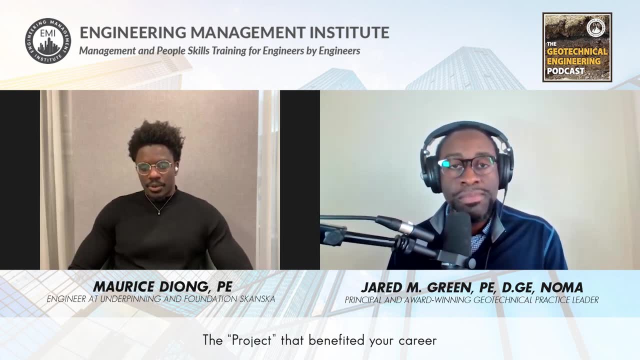 I'm just on my side And you know the inspector is doing your own thing. No, We want the job done, We want it to be done well. So in this instance I work with the inspector. for example, Greg Lucky, really smart guy. 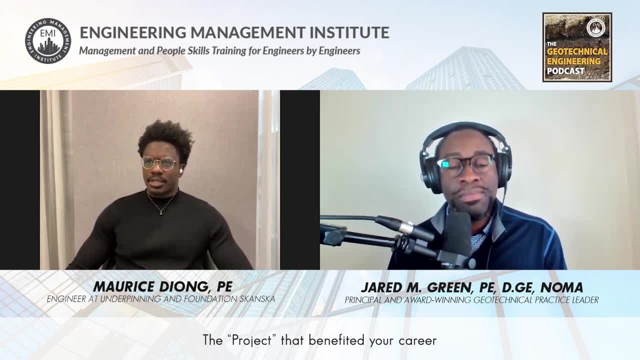 He would, of course, check everything we do And sometimes, when there is a certain issue, we would all get together and try to find a solution. right, And that's something that I think we have a tendency to forget: that, hey, we're all part of the same team. 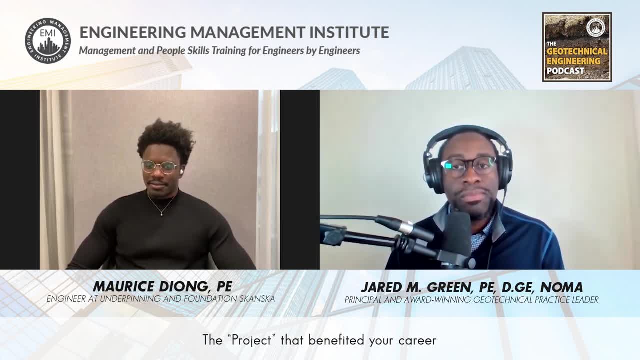 Yes, different parties, but we all want the job done, safe, right, And we want it to be done well. And we want it to be done well. What else? Oh yeah, Another thing I would mention from that I got from the job. 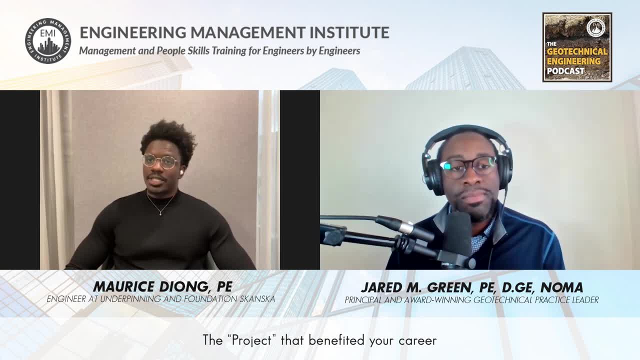 is how much knowledge you actually find in the field. So, as engineers- yes, we went to school for that, But experience is very important, right, And a lot of time. we have ten and 16.. We have to neglect all the people in the field. 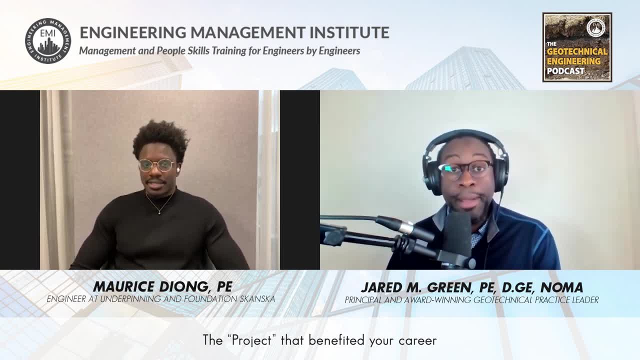 But I mean, that pool of knowledge is just massive. So I would spend time talking to our foreman, Mike Miller, And I'd tell him: hey, this is what we want to do, But I don't know, I don't know if it's possible. 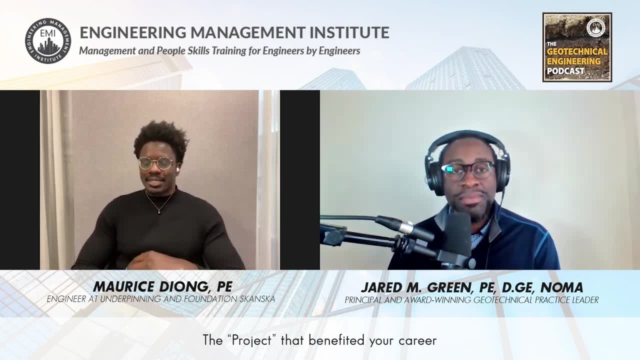 And he's like, well, just get me this and do that. So I think we need to spend more time talking to engineers, to the people in the field, Because, at the end of the day, I have five, 10 years experience. 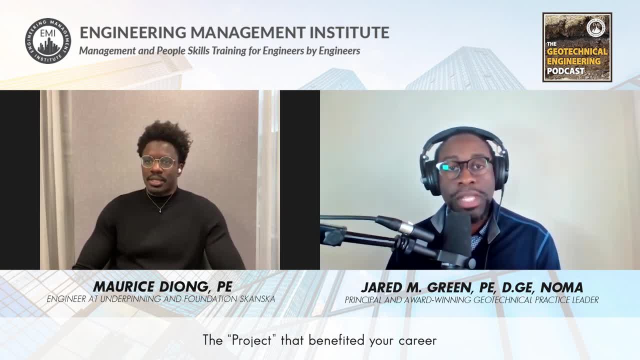 But that person has been doing that for 20 years. It's very important to talk to them. Yeah, I mean that project, from the design to coming up with some specific custom-built rigs. it was crazy. You get there, Honestly. you get there. it's daylight. 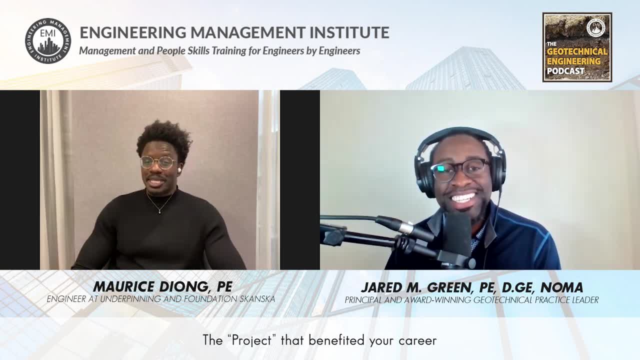 And by the time you get out, it's night, Because you're in the basement. you never see the sun. It was mad. Yeah, It's a good feeling when you're working on something. when it's nothing, You're putting together calculations. 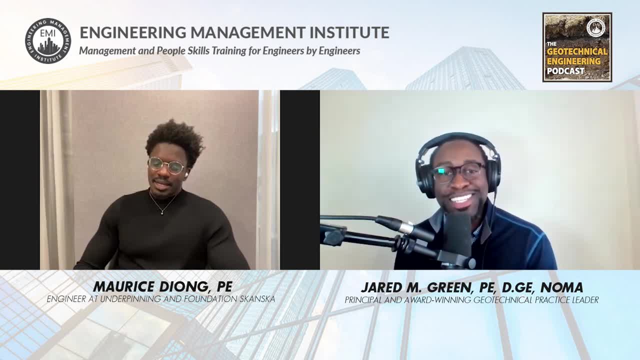 And then you're actually figuring it out in the field. It's a good feeling. I'm not going to lie. It was so hard. at times I was like maybe it's time for me to retire, Like I don't know, what am I doing? 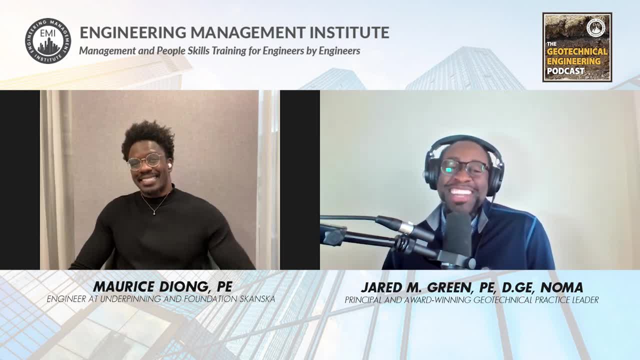 But it's got to be done. Yeah, Got to be done, Got to be done, Yeah. So what kind of things change? You get to the field and things have changed. What's changed? The logistics And what kind of things change? 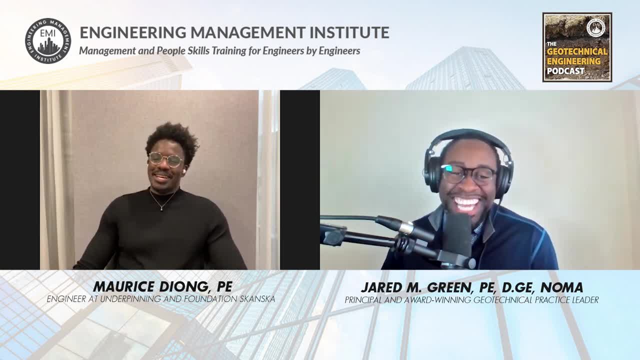 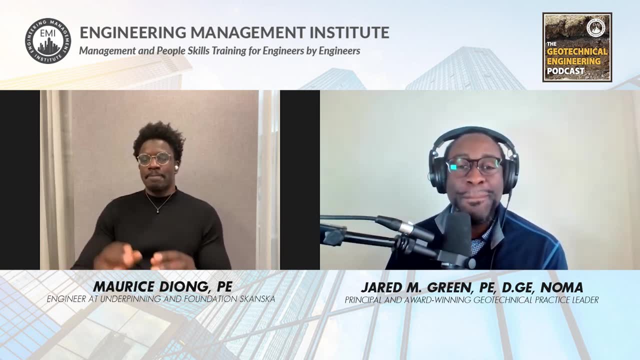 I mean everything, Everything, Everything. OK, so this is the thing, And again, that's the importance of planning Right. So we have a long-term goal, We know what we want to do. It's all the files. 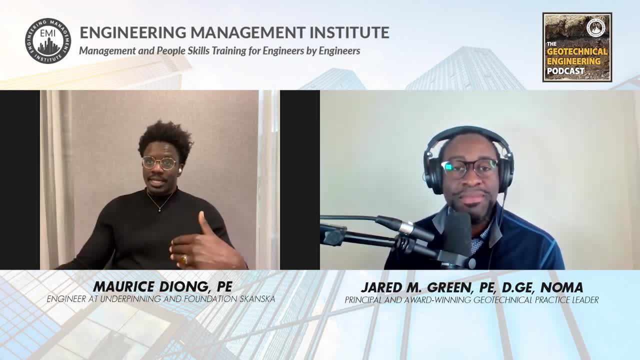 Then we have some milestones, We have weekly goals, And so what we would do, Matt and I, would sit down and then plan for the entire week By the end of the week. this is what we have to do so that the other crews can keep working. 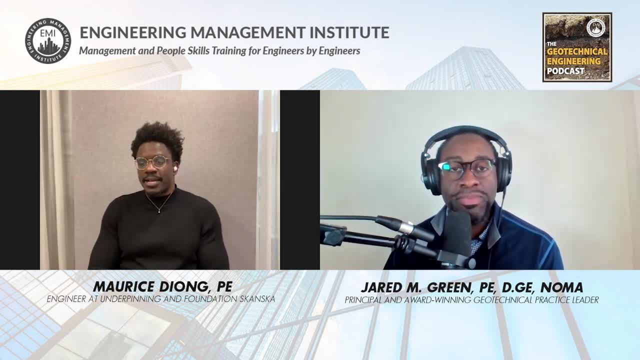 Because, at the end of the day, cost is a driving factor. So we would come and we'd spend the whole time planning. Actually, we would even plan every day. So we would plan for the week and then we would plan every day. 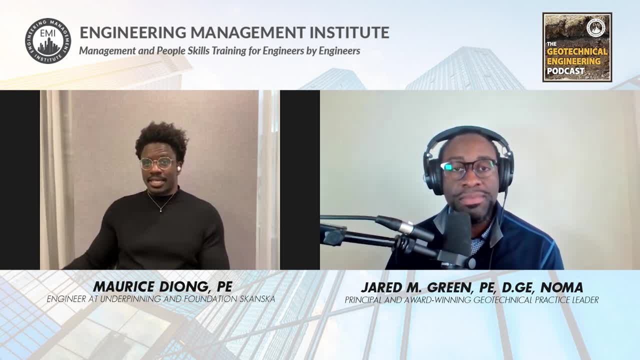 OK, tomorrow. this is how we're going to do it, This is what we're going to do, This is how long it's going to take, And then you get there in the morning and the super tells you: well, I think that's a good idea. 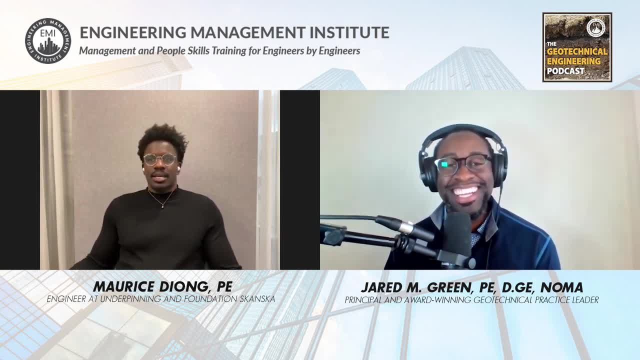 but we won't do this today. We don't have time, We're going to do something else. So the whole week, the planning that you did- yeah, it's gone. OK, what do we do now? Or sometimes, something, really. 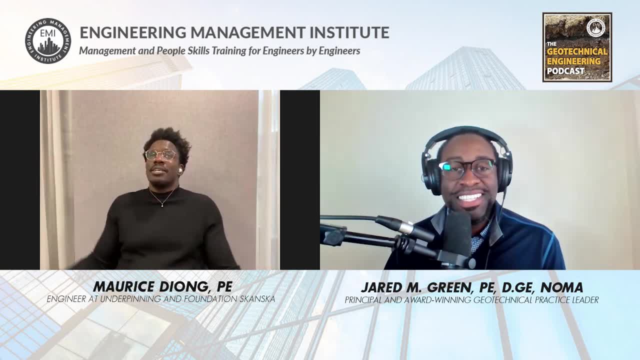 You know, some crazy stuff happened. You have 12 feet of headroom, And sometimes you have less than that, And it's just impossible. So what do you do? No, you have to stop everything and then come up with an alternative. 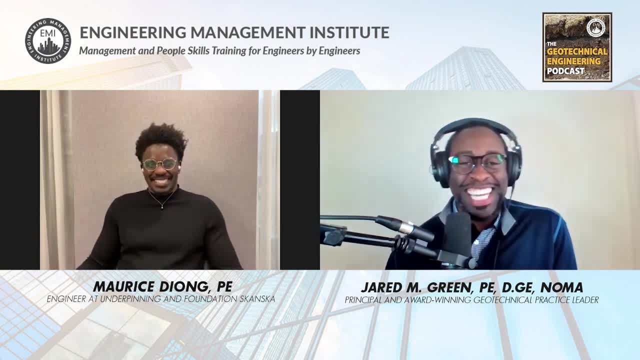 Ah, You see, just thinking about it, Thinking about it is kind of stressful, right, Yeah. So yeah, kudos to John Savera and Sons, that company, I mean they did great Yeah. And kudos to honestly all the crew, the laborers, the foremen. 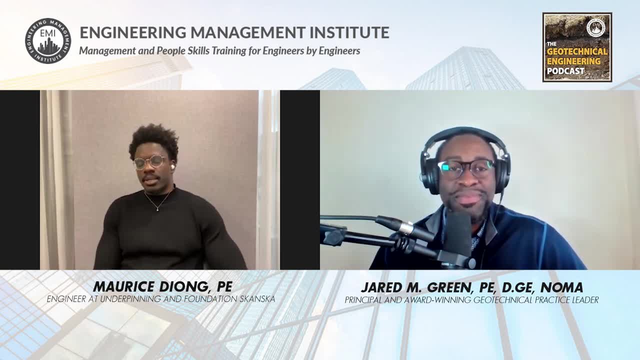 the operators, man, all really smart and talented people. So it wasn't easy, Yeah Well, yeah, One of the things that was- I don't want to say nerve-wracking, but one of the things that was a big eye-opener for me. 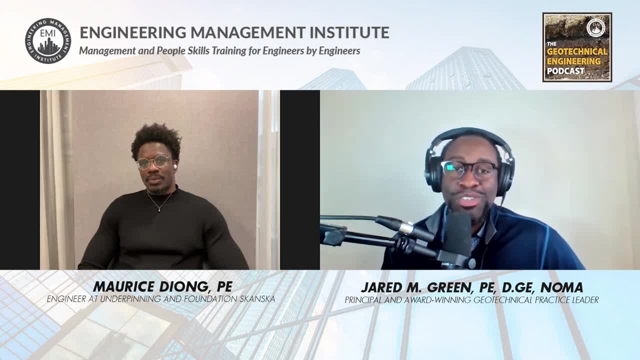 early in my career was just seeing that you could design something, but there's so many different parties that are a part of that design being implemented. So you have your specialty- foundation contractor, You have your excavator, You have all the trades associated with that. 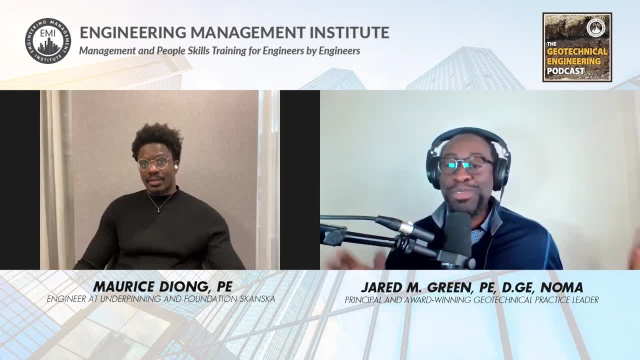 Your general contractor. In some cases, maybe demolitions happen at the same time, So there's a lot of pieces And trying to put that all together is crazy, You know. I'm glad you mentioned all of that, because it all happened at the same time. 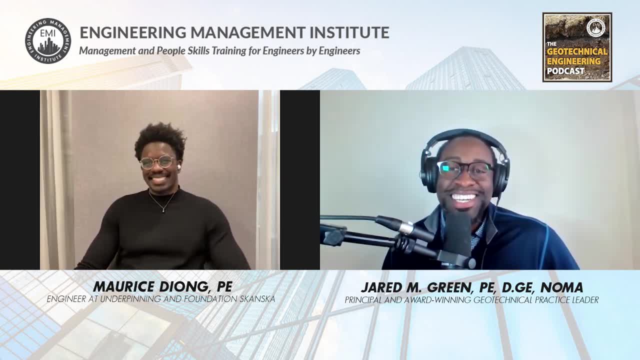 Oh my goodness, Yeah, Yes, it did. Yeah, Oh man. Well, Maurice, you know, when you think about engineers and engineering, there's always this focus on getting things right, And sometimes you can have this obsession with obtaining professionals. 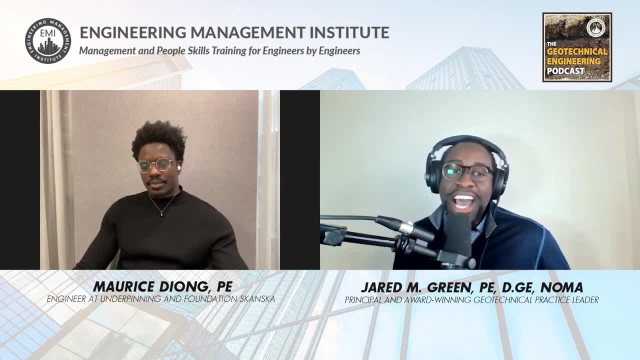 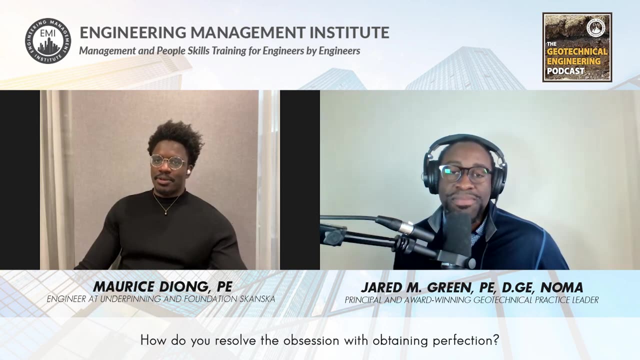 Mm-hmm, Mm-hmm, Mm-hmm, Mm-hmm, Perfection. How do you resolve this? How do you resolve it? Well, I think I have to start by saying that life is essentially imperfect. 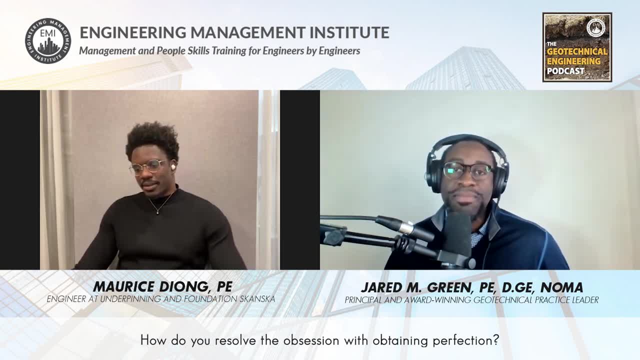 right. But when it comes to engineering- I was talking to a friend yesterday And we agree that the stakes are higher. You know, we can't just go halfway Right. we have to do it right because, uh, people's lives are at stake and you know, i think what's what's? 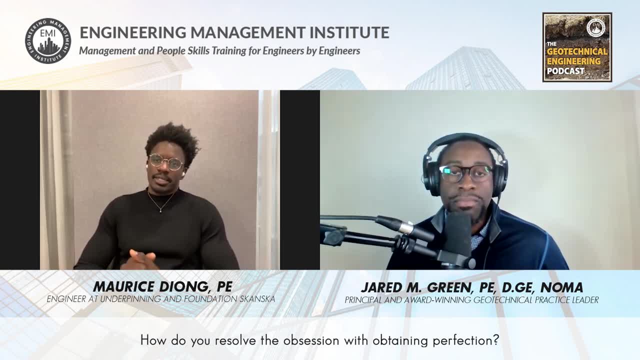 important is. i think that's also why we have tolerances. uh, you know, like we want it to be perfect. but then, uh, you could do a design, for example, of, uh, let's say, four foundations. you have different loads, so now, what are you going to do? you know, ideal scenario would be: you have 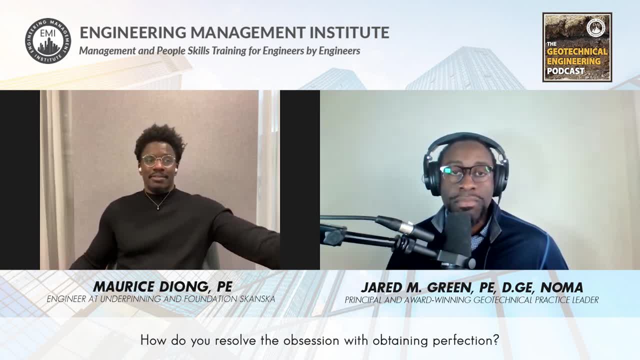 the perfect uh size for a given load, but you're not gonna end up having 20 different uh designs for you know. so, okay, what i'm trying to say, i guess, is it's important to remember that. you know we have to be practical uh, we have to be safe and we have to be uh, and that cost also, you know plays. 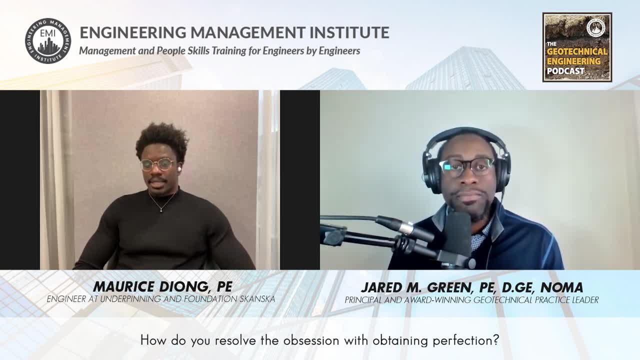 a big role in what we do, um, and when it comes to perfection. i remember back in college, we were talking about, i think it was a geos, yeah, so soils mechanic class. we were talking about, uh, consolidation, i think it was a time rate consolidation, and so they show you this graph and they tell you that at, maybe within you know. six months you reach 90 consolidation, but then for you to reach the remaining 10 you take you maybe an additional six months. so, yeah, maybe that that hundred and you never get actually 10 right, a hundred percent. so that extra nine percent is it really worth all that time all? 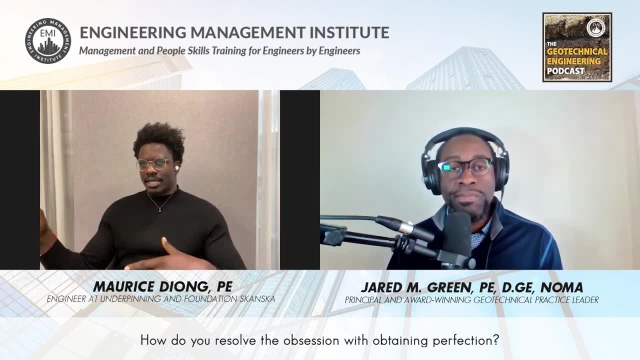 that money, you know, like, what is perfection? is it getting to that 99? or is it really, when you take all these different variables into account, uh, you know the most effective solution. maybe that's what perfection is: not always focusing on one item, you know, because in our industry there is a lot more variables involved. yeah, you're absolutely right. and if you 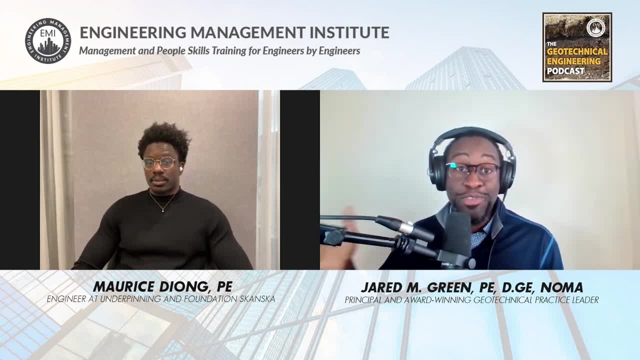 kind of lose sight of the big picture. you can miss that. you know you're fighting for that last fraction of a millimeter and it might not make a difference for the overall project. you know, yeah, in some cases it may, but in other cases it may not. so it's like you know you have to make sure. 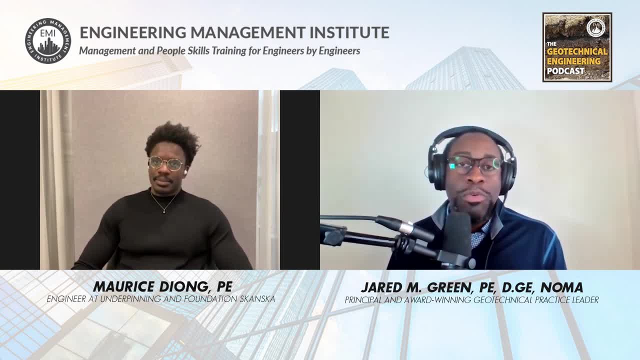 you're thinking about that, that's true, yeah, excellent. well, before we take our break, is there another, let's say a final, piece of advice? you want to give engineers to the listening out there? well, i would say, uh, you know, to take advantage of all the resources. 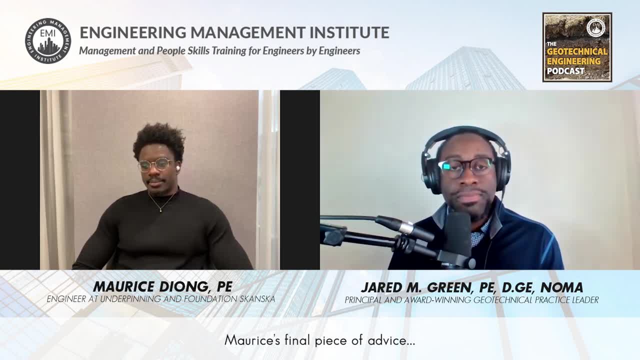 that are out there. you know, um, when it comes to our industry experience, it's very important. but what? what is experience really? you know people think of it, as you know the amount of time that you spend, you know, doing a task like, oh, i've been, uh, i work, in construction for like 10 years. yeah, 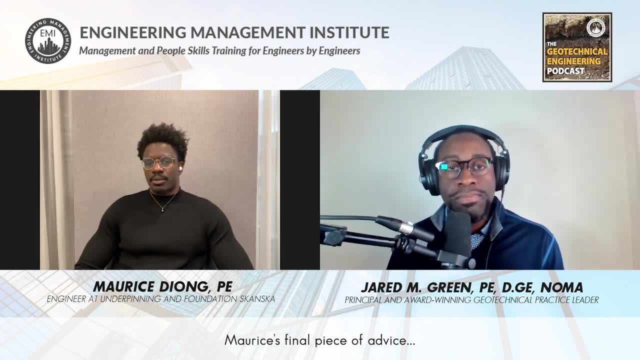 but what does it really mean now? what have you done? so yes, i can say, like you know, i'm an engineer, i'm a in my position, i can stay maybe 10 years and you know, yes, i'll have some experience. but i can also go and and tap into, let's say, a deep foundation, for example dfi or adsc or ase, you know, and build. 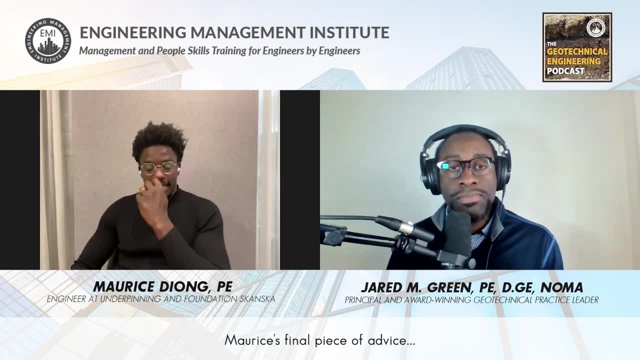 a network. um, like i said the other day, i i reached out to, uh, donald bruce, right, i just email him and i call him, and then here we are, talking about my profile. i mean, that's something that would have taken me maybe an extra year to learn and i learned all that stuff within 10 minutes, right? 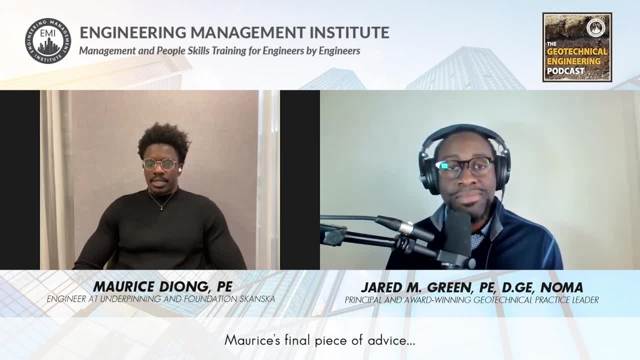 so just remember to. you know, uh, yeah to to build a network. you know, uh, you're not alone. there's a lot of people out there and they want to share, you know, so, take advantage of that. um, yeah, that would be my, my piece of advice. so that's great, that's great. the reality is that you know, we're. 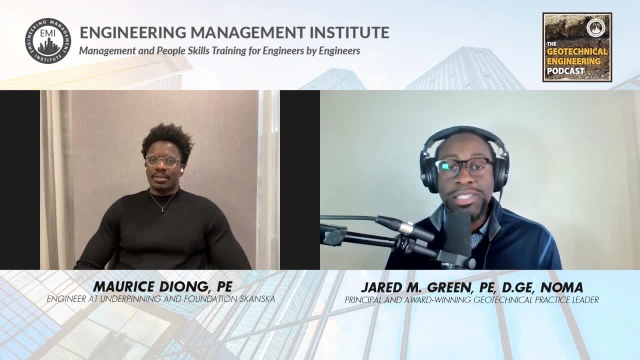 part of an industry where people want to help. it's very rarely you're going to reach out to somebody and say, no, i can't help you with that. so that's a great piece of advice. great piece of advice. so we're going to come back in just a 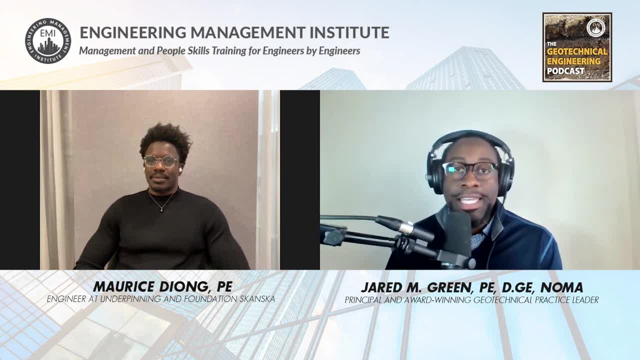 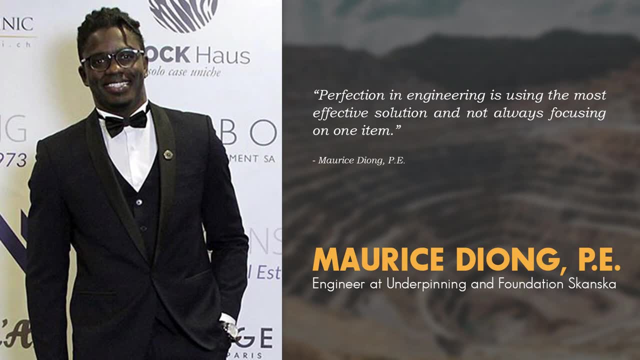 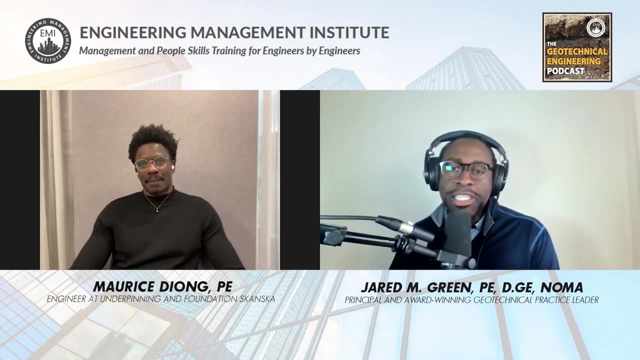 moment and we're going to close this one out with maurice and our career factor safety end segment. stick around, welcome back. it's time for our career factor safety end segment. in geotechnical engineering, just like many disciplines of engineering, it's important to incorporate a factor of safety into 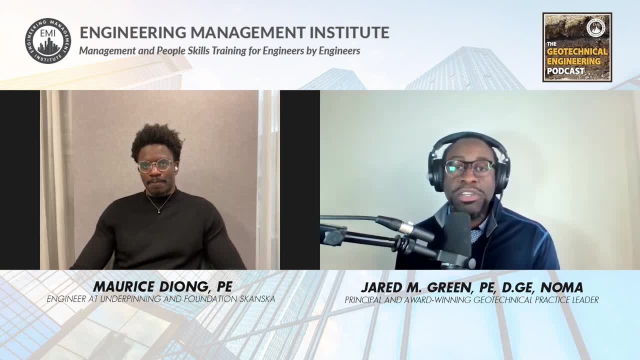 your design, but what about incorporating a factor of safety into your design? today, of course, we're speaking about maurice young maurice. you've already had a successful career and you're still in your career, of course, but when you look back at your career, what's one? 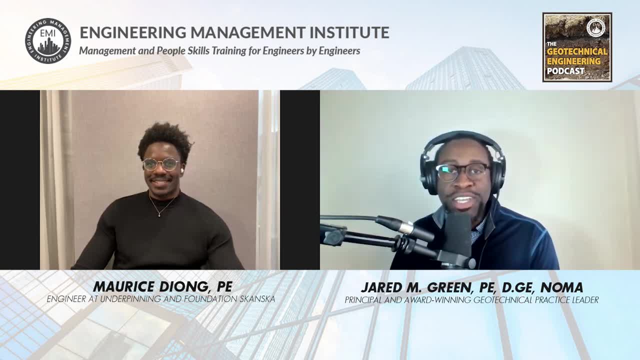 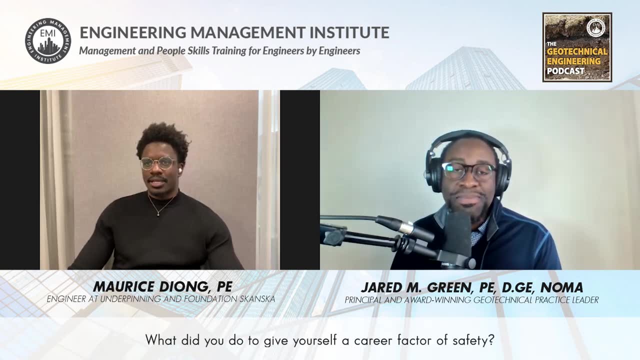 thing you've implemented in your career to give yourself- let's call it- a factor of safety in your career. well, um, let's say, i think the first thing that comes to mind is i've always been up for a challenge. you know, uh, when certain assignments come, i'm not necessarily excited about them, but 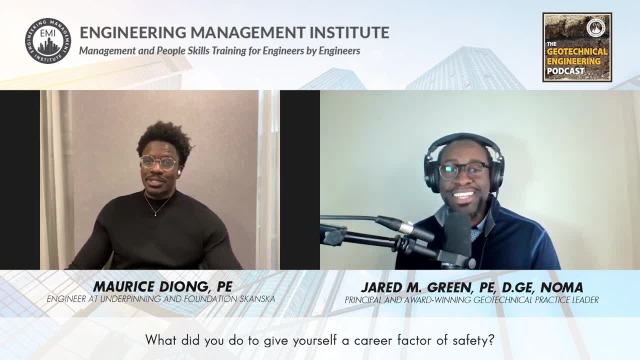 you know, i just want to say thank you for your time and i'll see you next time. and you know, i give it a try. give it a try, uh, like like my mentor, uh, jim reilly, would say: i'll do what i have to do and i'll do it gracefully because i'll do it anyhow, right? so 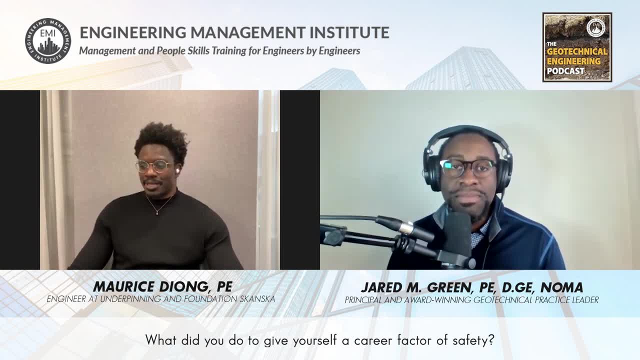 that's the mentality i use. i go and i just do, uh, you know, whatever they throw my way, and you know i give it a try first. um, the other thing i would say would be so, although i i specialize or focus on, uh, you know, in-house. 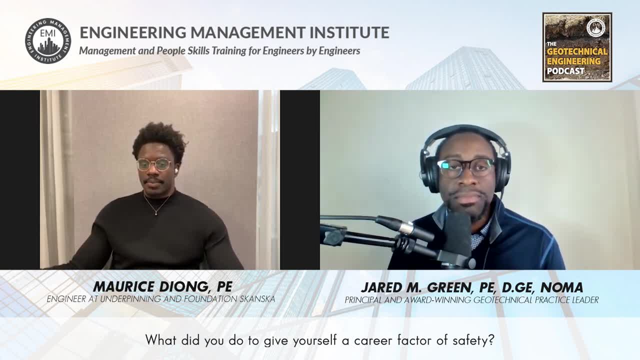 design or in-house engineering. i also spent some time doing other things, like you know, field engineering or, um, you know, estimating. so i'm somewhat well-rounded, you know, and- and i think that gives me an edge, like let's say, uh, you know, they know that i can do, i can do pretty much you. 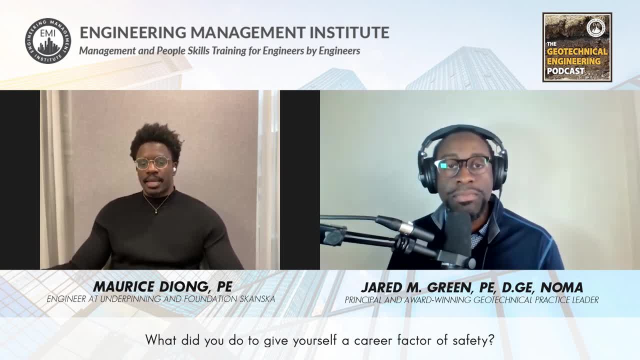 know i could be involved in a lot of different departments and, and i think it's also important, when you are, uh, when you specialize on one thing, i think it's important to know a little bit of, you know, everything that touches on that thing. so you know, uh, i think it makes you better. so i think 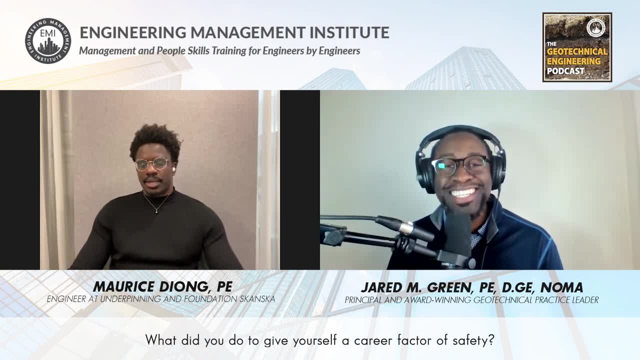 that was, uh, that's part of my safety factor, but ultimately, i'd say i don't think about it that way too much. but i think, uh, you know, if i think the answer is around the following question: right, if you were to leave today, how would that impact your company, right? if you, uh, if you realize that, hey, if i. 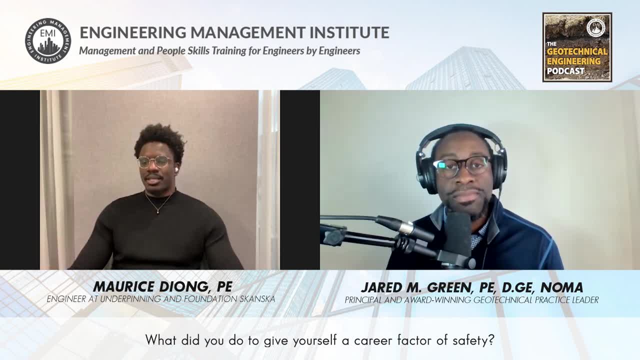 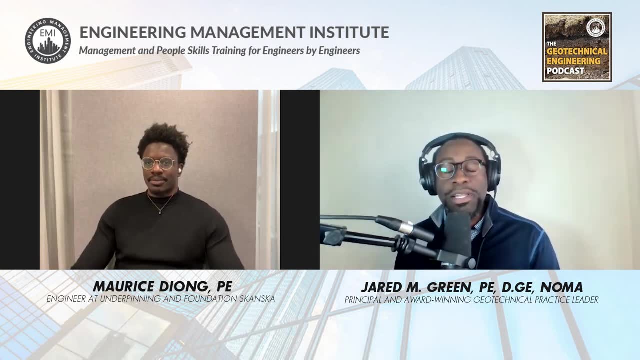 leave today that company. you know it's gonna affect the company greatly and know that you are an asset and i think that's the greatest safety factor that you can. honestly, i like it. i like it well. thank you so much for sharing that there. there's uh great stuff there for. 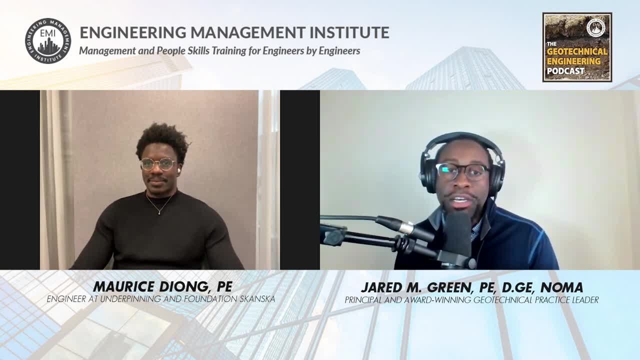 those that are listening and i appreciate you sharing that and, um, i would like to thank you for that. thank you for sharing that. you know the advice that you shared was great, not just for people starting out in their career, but, you know, seasoned professionals, so thank you for that. if somebody was listening and they want to reach out to you, what's the best. 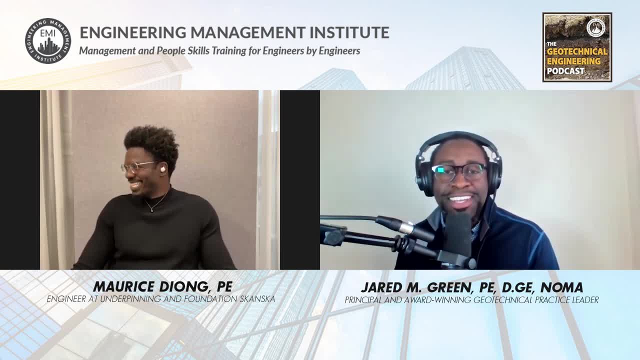 way for them to find you on social media or email you want to share. maurice, yeah, i'd say come find me at the foundation institute. no, but uh, i'd say, yeah, i have an email. so it's emily maurice. okay, d i o n. 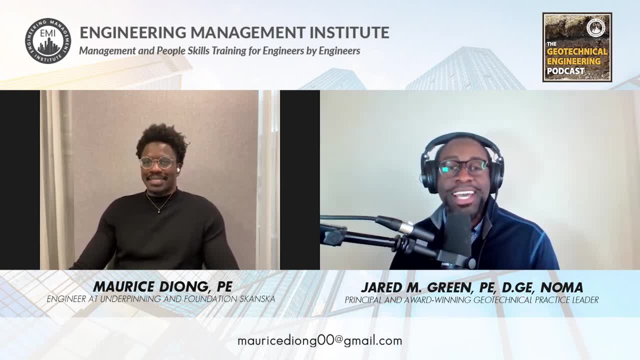 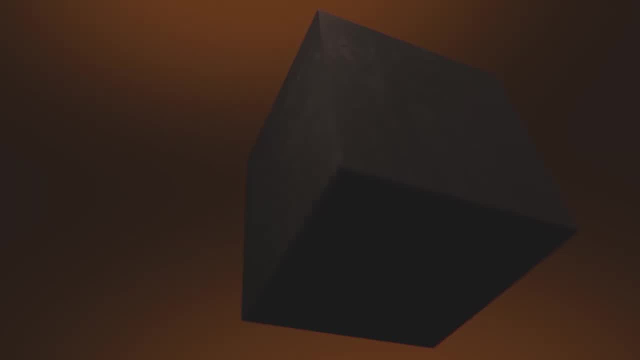 g. my last name, zero zero at gmailcom. excellent, excellent. we'll make sure we have that in the show notes. well, thank you so much for coming on. this is a lot of fun, man. thank you for having me. i hope you enjoyed the episode today. we would love to hear your feedback, comments and or questions. please feel free to go to.